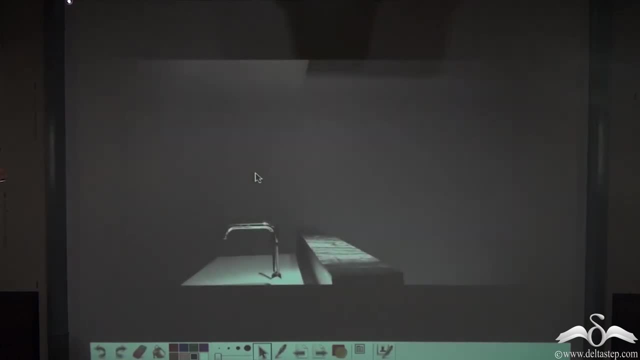 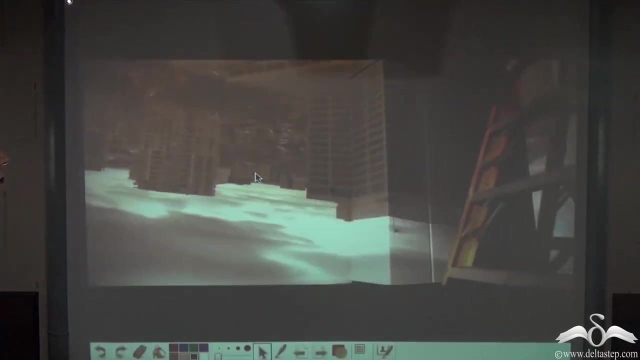 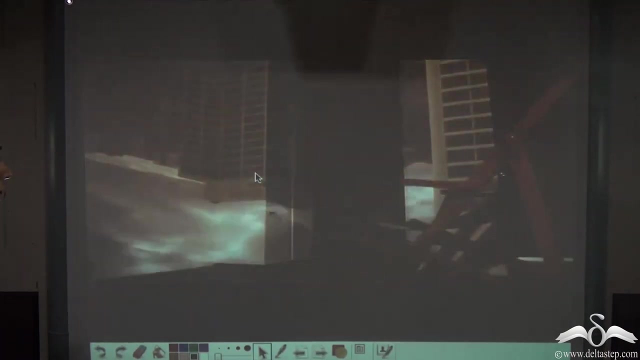 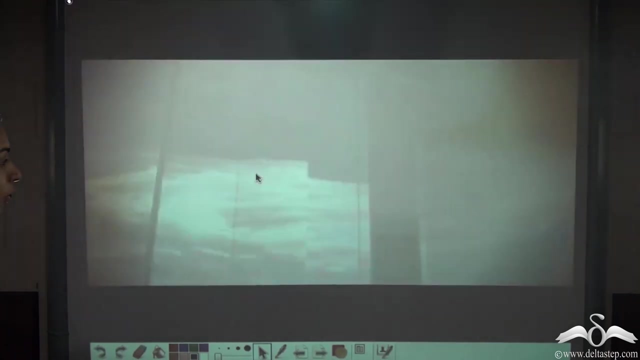 that is coming inside The house from that hole. Hey, what is this? There is an image of the surroundings of the nearby buildings inside the house. Wow, amazing, isn't it That man from the hole he created the image of the surroundings inside the house, which. 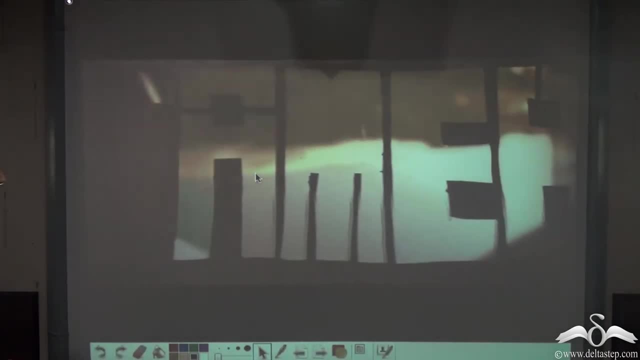 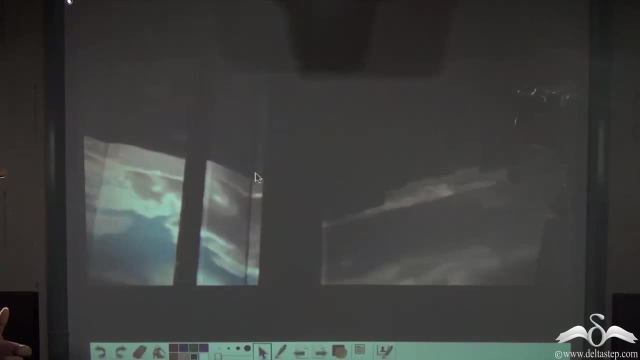 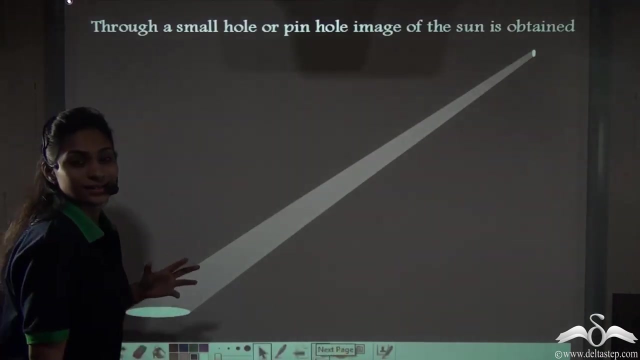 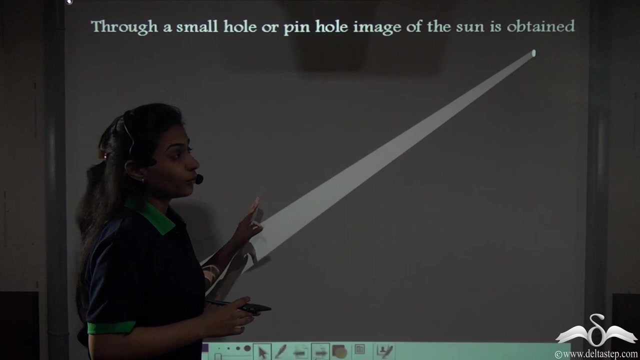 was in complete darkness, Though the image is inverted, but you can see everything that is outside without even looking outside. Ok, Bro, image has been created through a small hole. Well, yes, this hole is actually a pinhole and it can be created as a camera. That is called a pinhole camera. Now, even if your 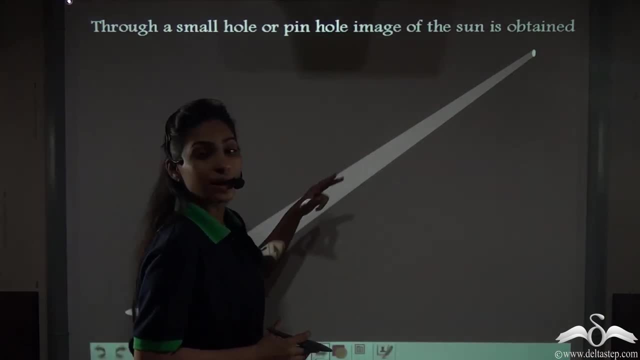 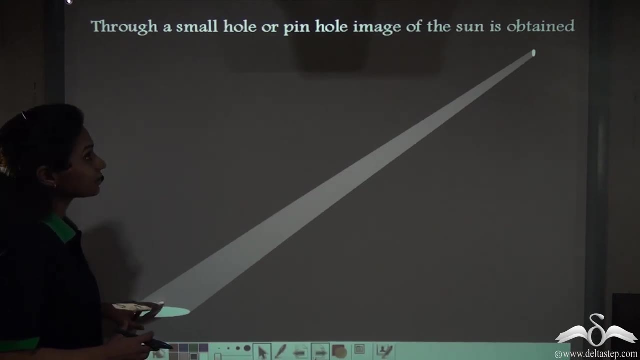 room is dark and there is a hole in your room from that sunlight passes in. Do you know what will create the image of the sun here? And this is why, through a small hole or pinhole, image of the sun is obtained. Now this actually acts as a pinhole camera. Now can we construct. 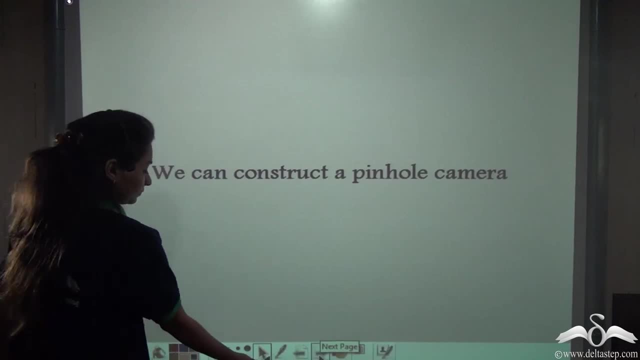 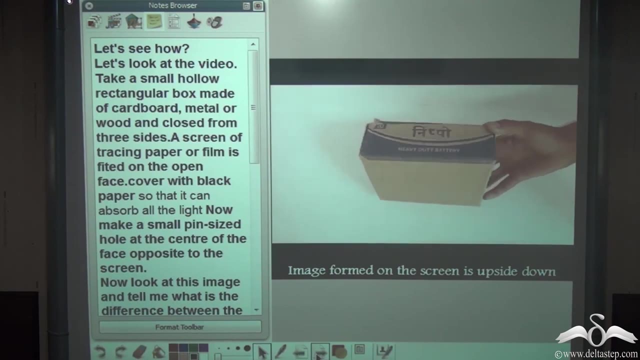 a pinhole camera ourselves. Well, yes, Take a small hollow, rectangular box made of cardboard, metal or wood and it should be closed, Closed from three sides. Now, screen of tracing paper or butter paper or film is to be fitted on the open face. So we have carefully placed the butter paper. 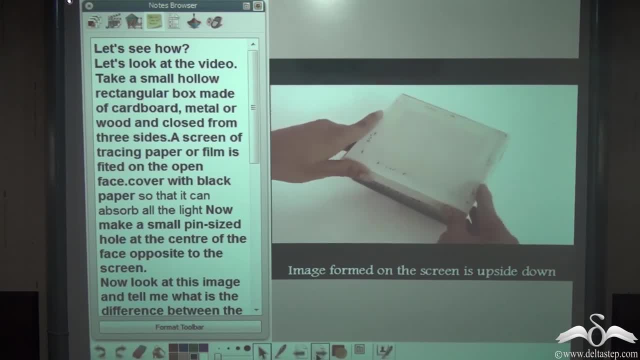 on the open face. Now we have carefully placed the butter paper on the open face. So I have carefully placed the butter paper on the open face. Now we cover the hole box with black paper So that it can absorb all the light. Now make a small pin sized hole. 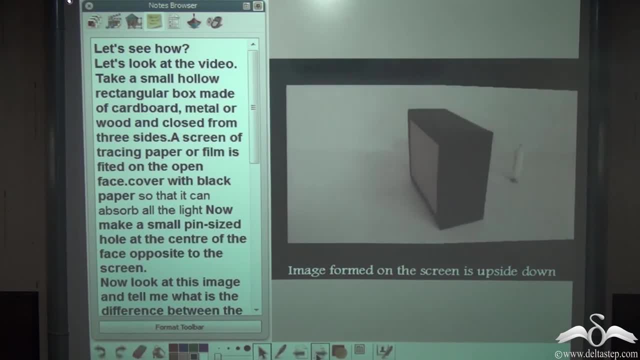 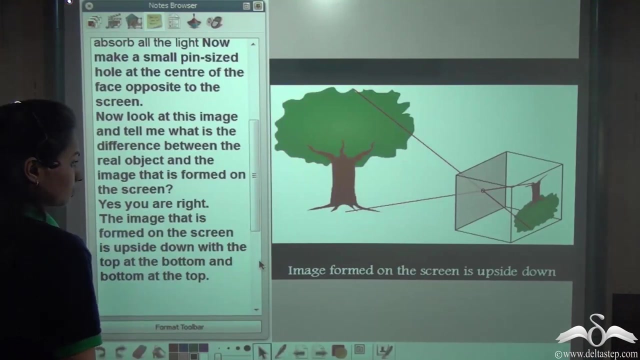 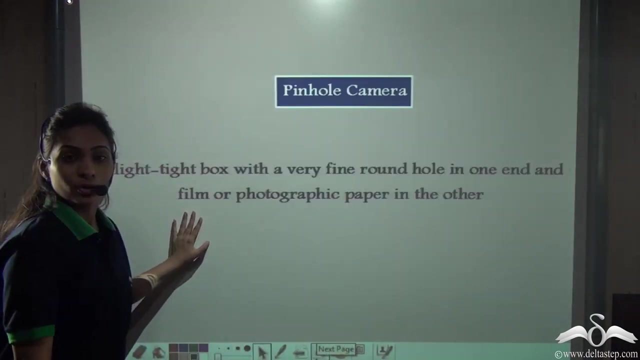 at the center of the face, opposite to the screen. Now, see, we will create the image of the candle inside the box. Well, see, this is the image that is created inside the box. See, it looks something like this. So now you know how to make a pinhole camera. 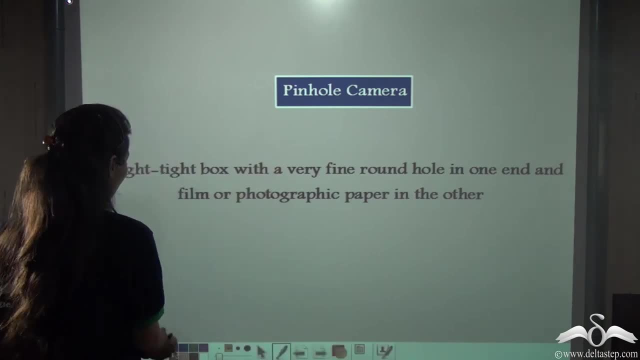 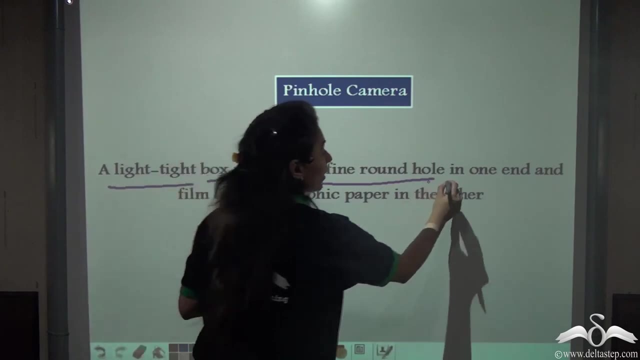 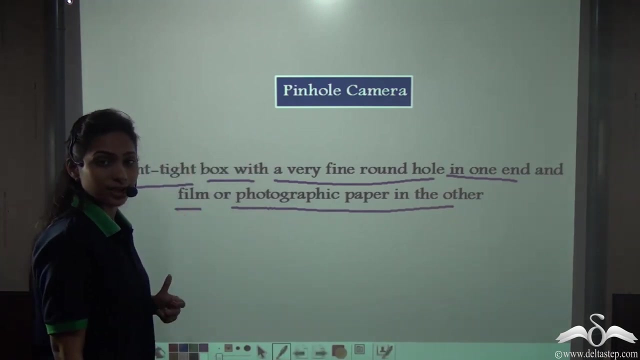 So what is a pinhole camera? Now, pinhole camera is a light, tight box with a very fine round hole. that is the small pinhole in one end And fill or photographic paper in the other. That is the butter paper that we have used in the experiment. 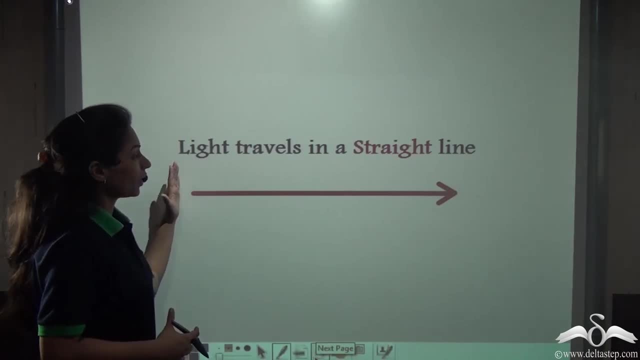 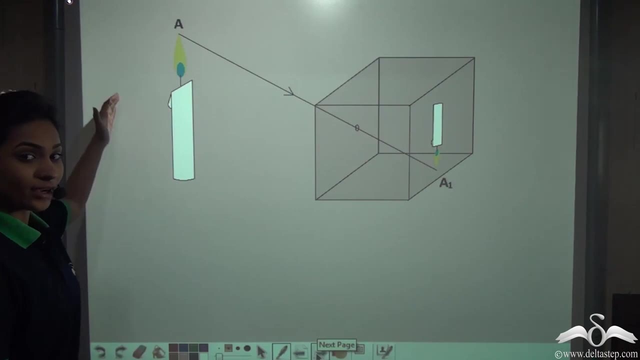 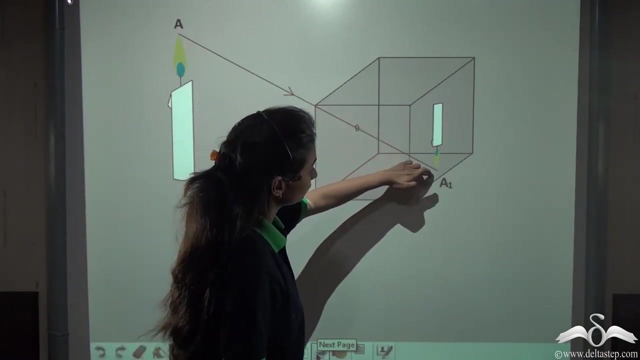 Now, how does this pinhole camera work? Let's see. Now we know that light travels in a straight line. So here light travels. so the light will travel from the point A. Light will travel in a straight line. Now it travels through this line. 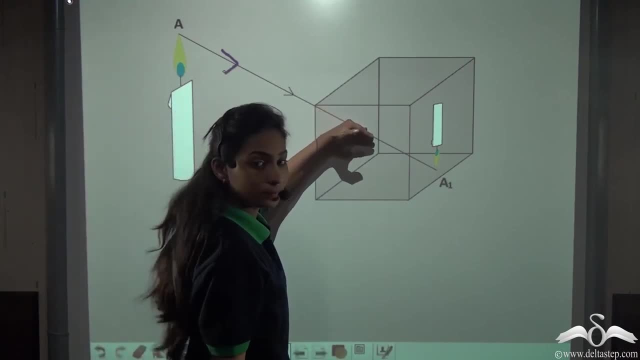 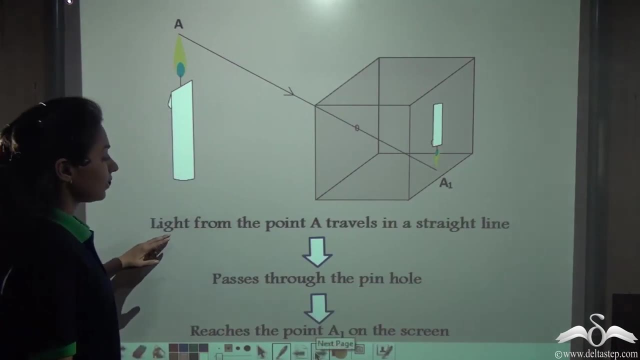 Now it will reach the pinhole and it will pass through that hole And it is reaching here at the point, say, A1. So we can say that light was coming from the point A and it travels in a straight line. Now, second, it passes through this pinhole. 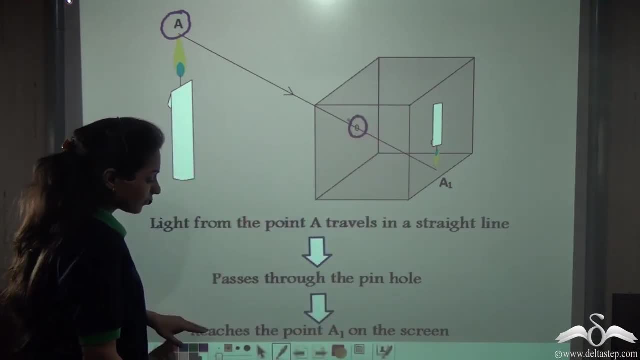 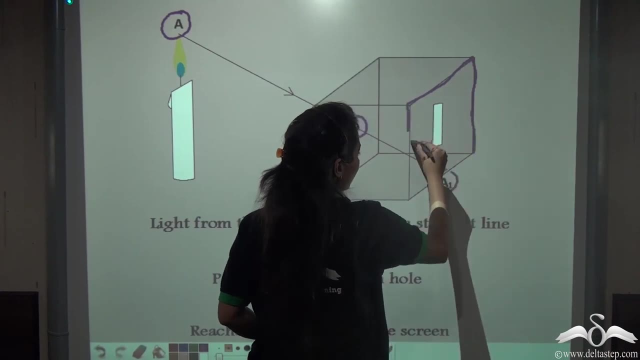 That is how the image will be created inside the pinhole camera And it reaches the point A1 on the screen. Now this is acting as a pinhole camera. This is acting as the screen of the pinhole camera, where the image will be formed. 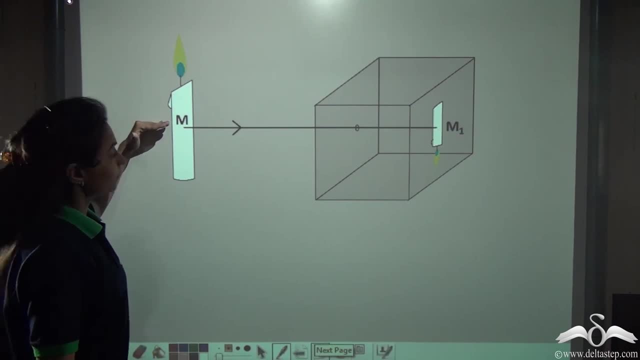 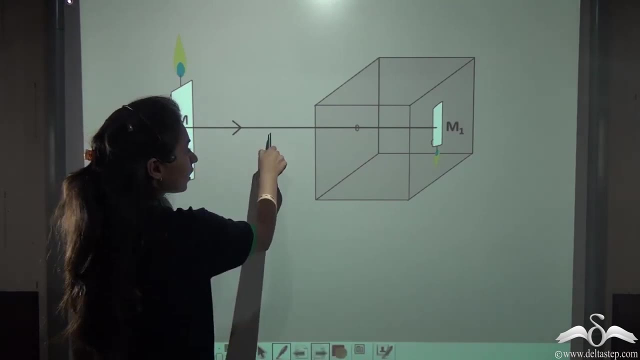 Now the second light that is here. the light rays are passing, So the light will pass from this middle part. Let's take this point as M, So the light will pass from the point M again in a straight line. So it is passing in a straight line. 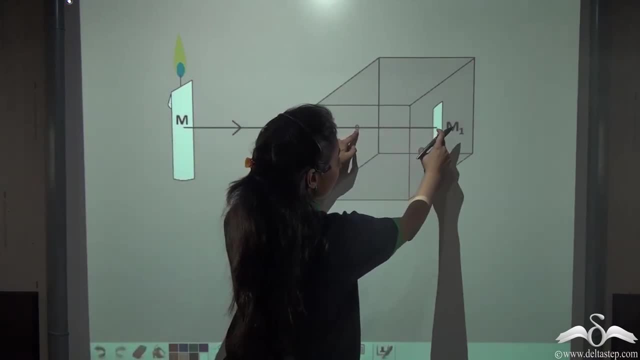 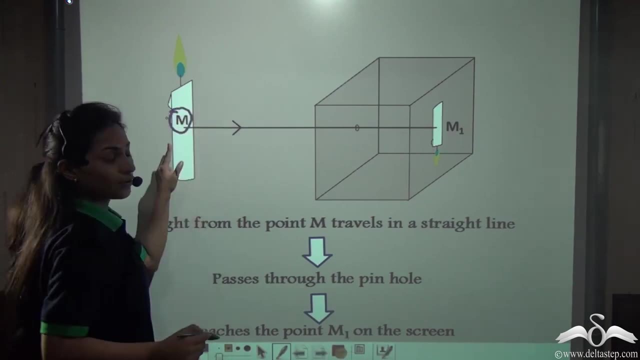 Now it is passing through the pinhole and it is creating an image here at M1.. So we can say: light from the point M travels in a straight line. Now it passes through this pinhole and it reaches the point M1 on the screen, which is: 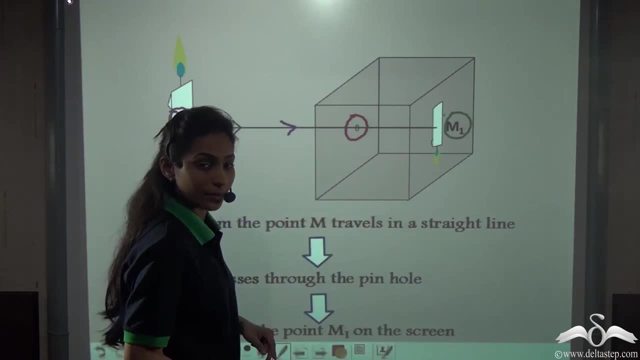 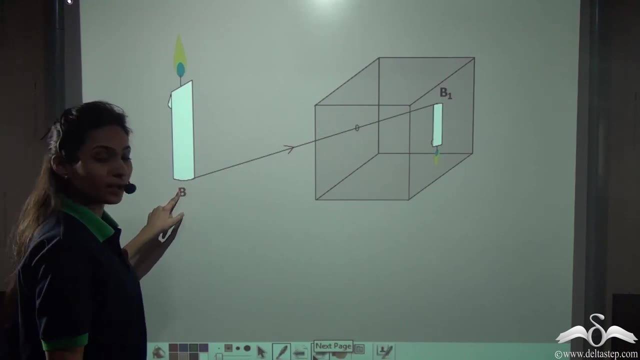 acting as a screen which is there in the pinhole camera. Now, the third thing is that the light ray passes from the point B so that it can complete the candle Right. So light from the point B travels in a straight line, passes through the pinhole and reaches 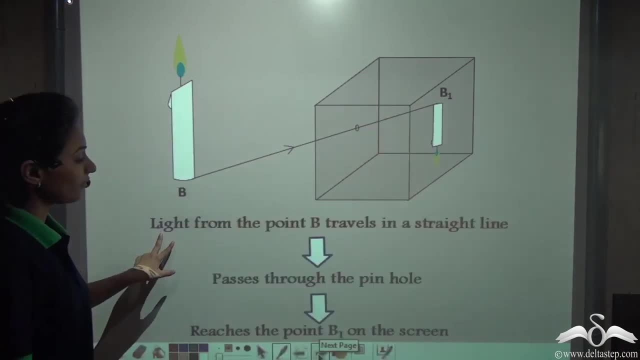 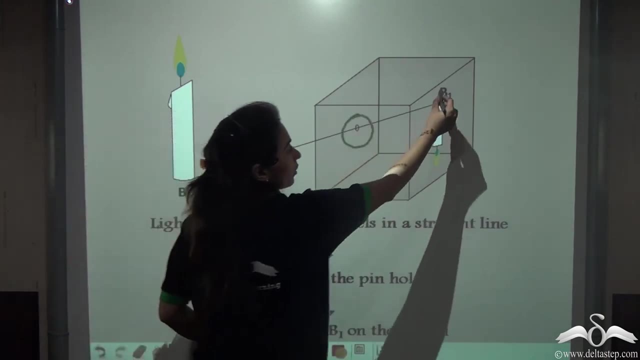 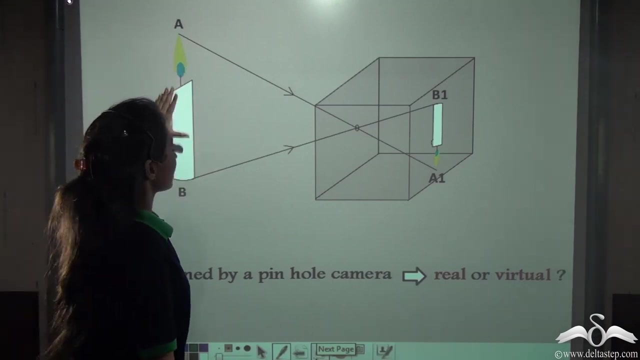 the point B1.. So light from the point B travels in a straight line. It passes through the pinhole and it reaches the point B1 on the screen. So you can see. this is how the image of this candle is formed inside this pinhole camera. 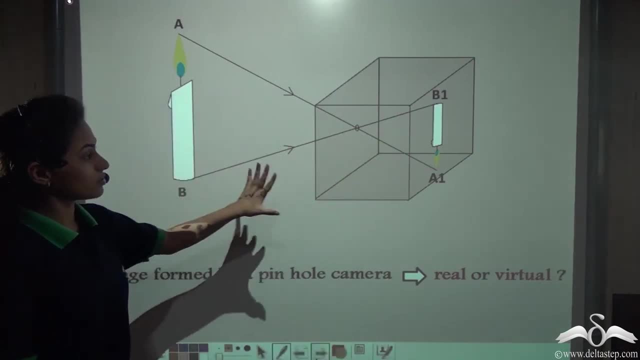 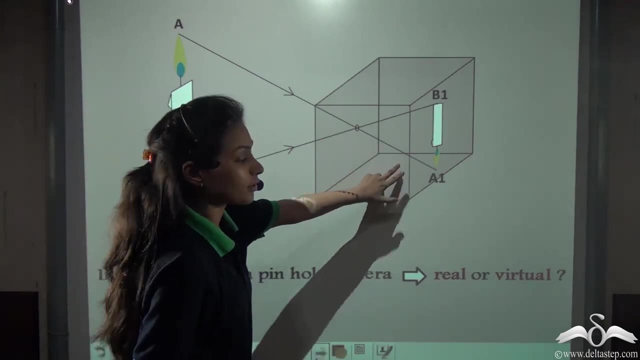 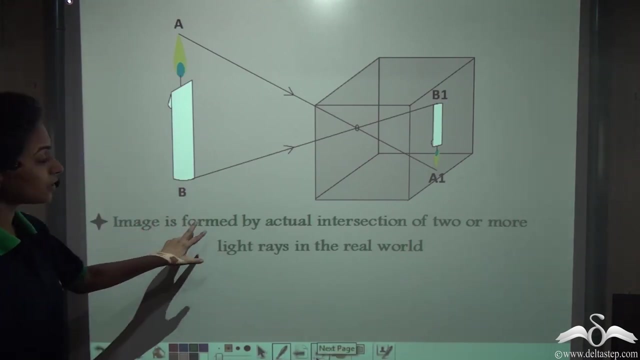 and we can see it. Now. you can see how the image is formed and virtual images. Now, can you tell me the image formed here? is it real or virtual? Well, we can say that the image formed here is by the actual intersection of two or more. 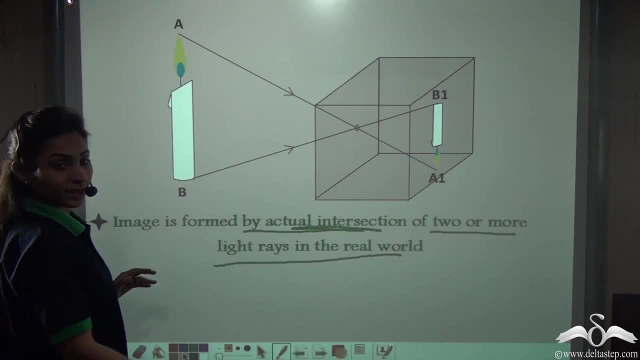 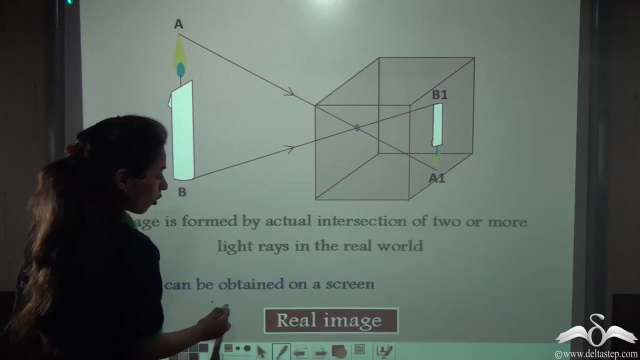 light rays in the real world. Here you can see that the light rays are actually intersecting in the real world. That is why it is what? Real image or virtual image? Well, we will see. Well, the image can also be obtained on a screen Here. the screen is here and we. 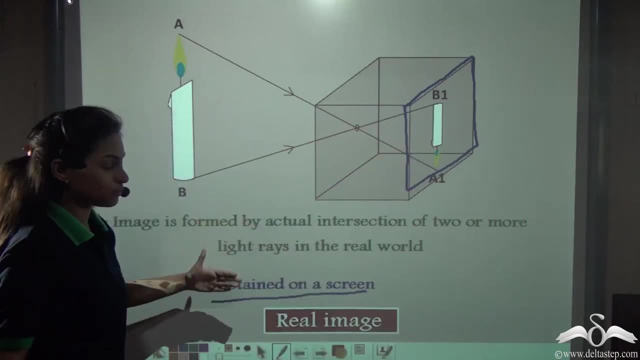 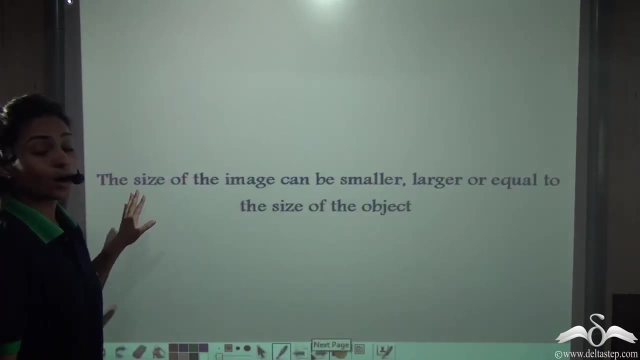 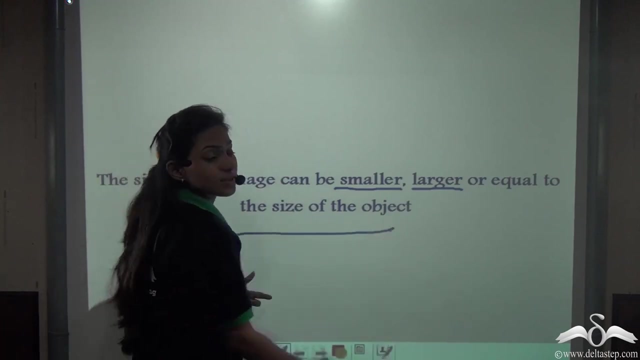 have already obtained the image on this screen. So obviously, both these points indicate that the image is a real image. Now do you know that the size of this image can be smaller, can be larger or can be larger. That can also be equal to the size of the object. Now, when can these cases take place? 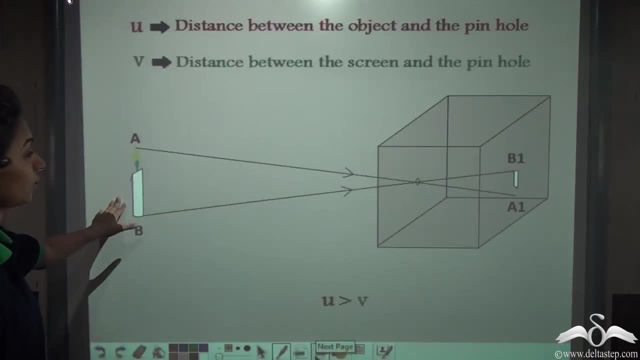 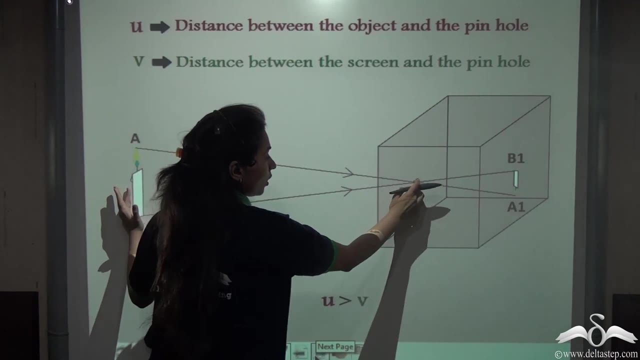 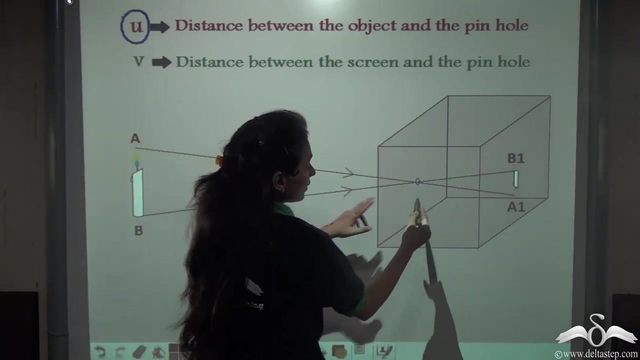 Let's see Here. we have assumed that the distance between the object, that is, the candle, and the pinhole is denoted by the letter U and the distance between the screen and the pinhole, that is, this distance is denoted by the letter V. 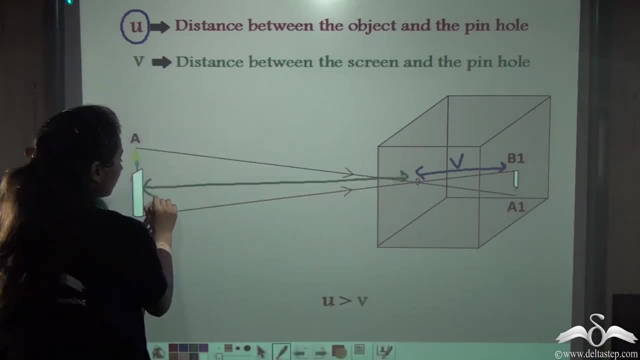 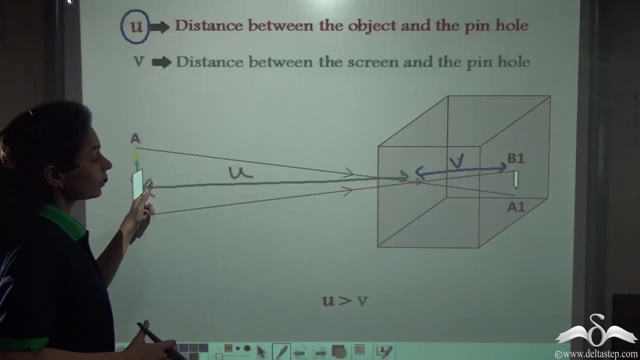 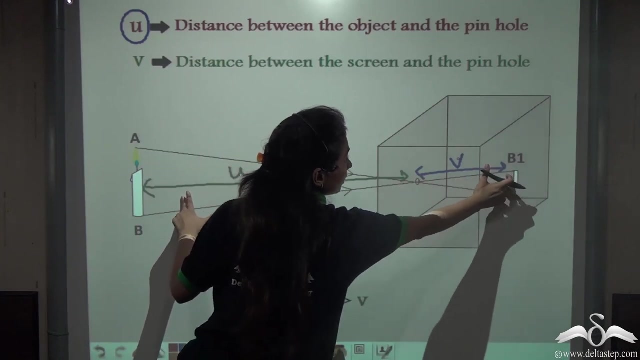 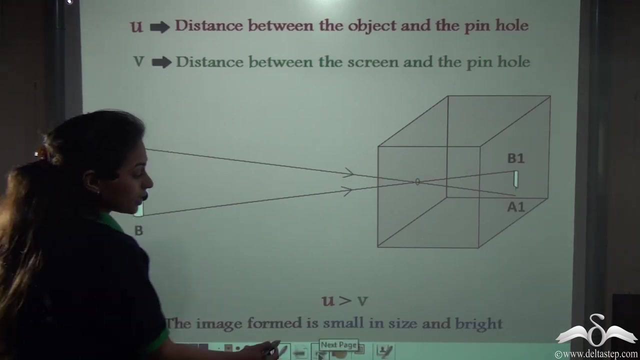 So this distance is U. Now, here you can see that U is greater than V. What does that mean? That the distance between the object and the pinhole is greater than the distance between the pinhole and the screen. So whenever this is the case, the image formed is always. 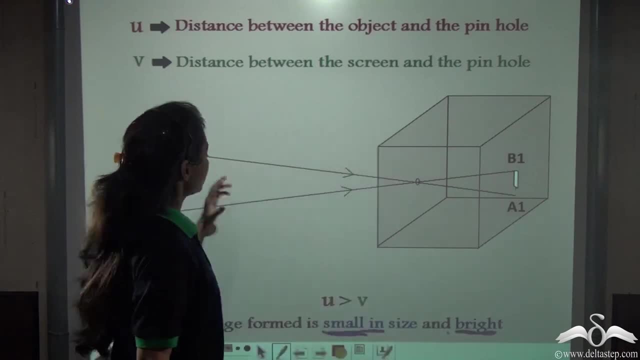 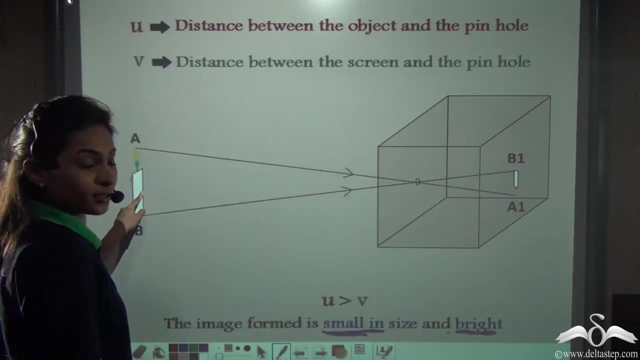 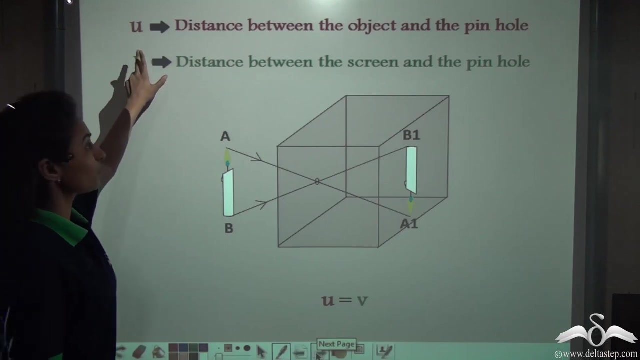 small in size and bright. So here the image formed can see that the image that is formed is smaller in size than that of the object and the image will be bright. Now, here again we are taking the case of u and v, where u is the distance. 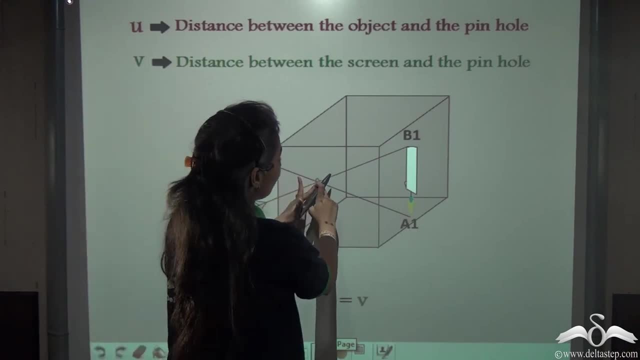 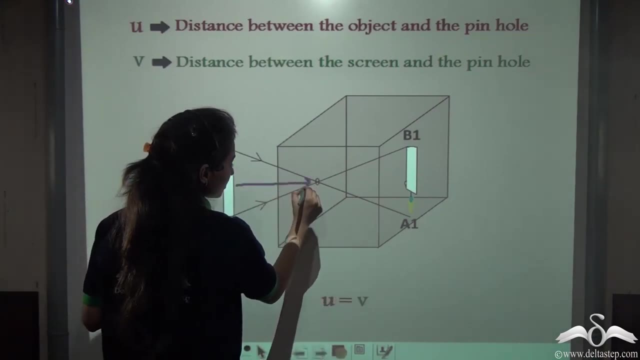 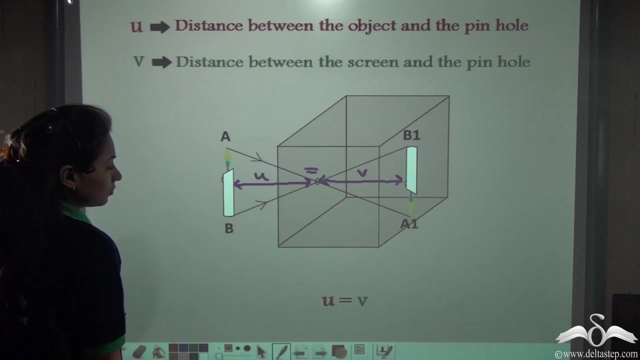 between the object and the pinhole, and v is the distance between the pinhole and the screen. Here you can see that both u and v are equal. That means this distance is equal to this distance. So in this case, what will be the nature of the image? Well, in this case, the 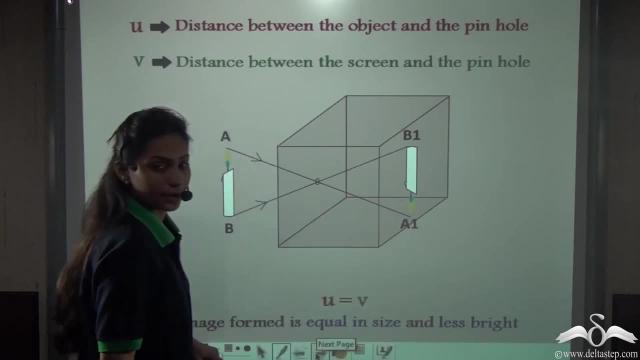 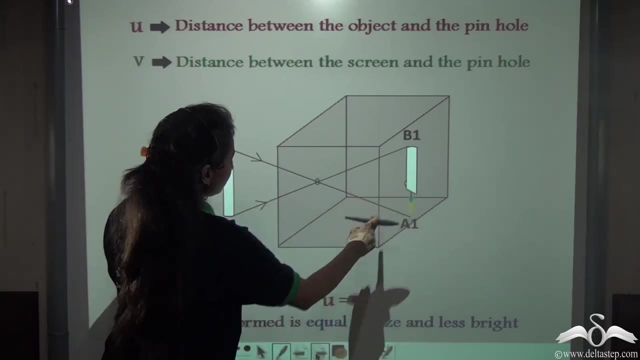 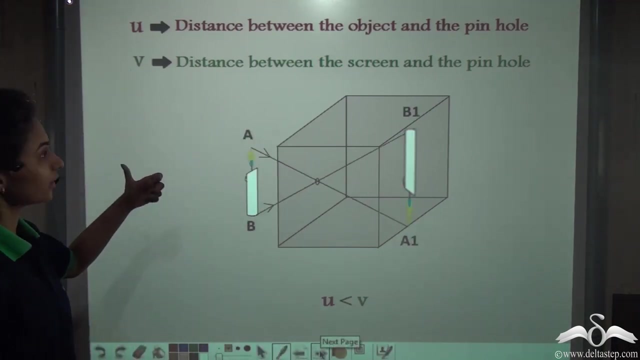 image formed is equal in size and it is less bright. Now you can see that the image here is at the same size as that of the object. this and this is equal. Now the image formed will be less bright. Now, again, we are taking the case where u is. 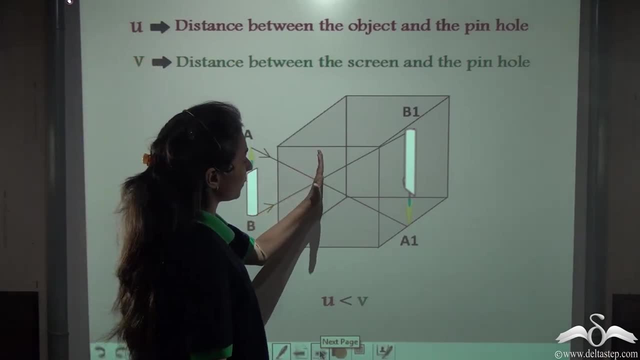 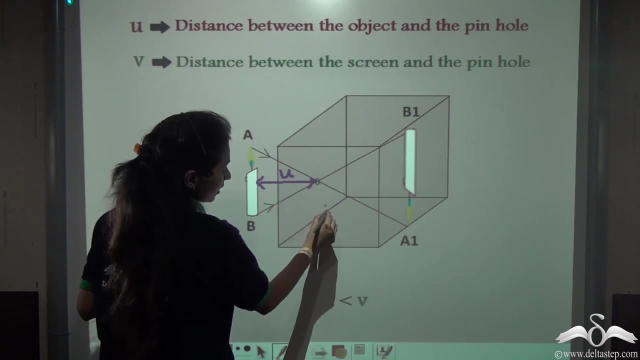 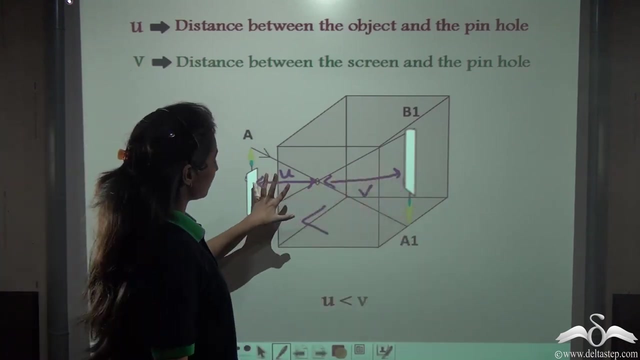 the distance between the pinhole and screen, and v is at the distance between the pinhole, between the object and the pinhole, and v is the distance between the pinhole and the screen. Here you can see that u is less than v. Now the distance here is greater than the distance. 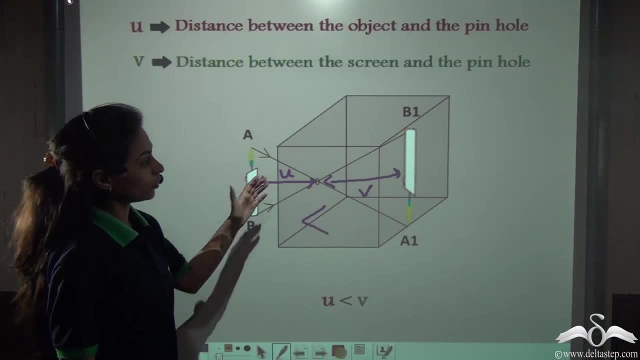 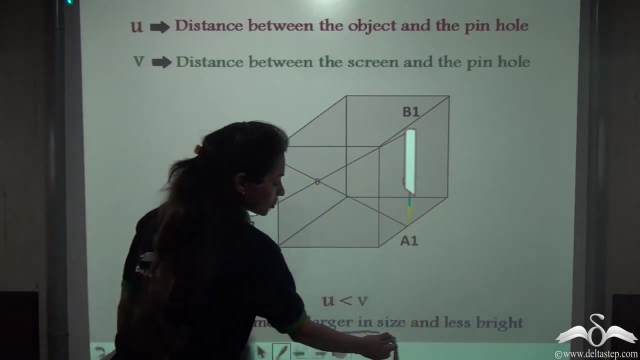 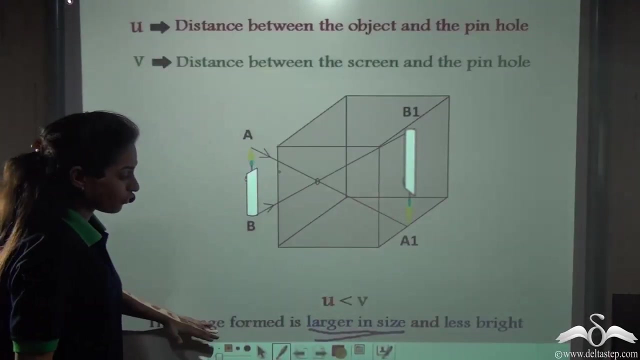 between the object and the pinhole. So what will be the nature of the image? You can make out from the image itself that the image formed is larger in size. Well, you can see that your self now, whenever this is the case that u is less than v, then the image formed will.